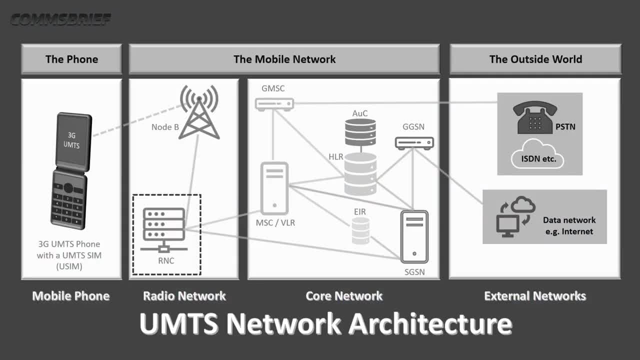 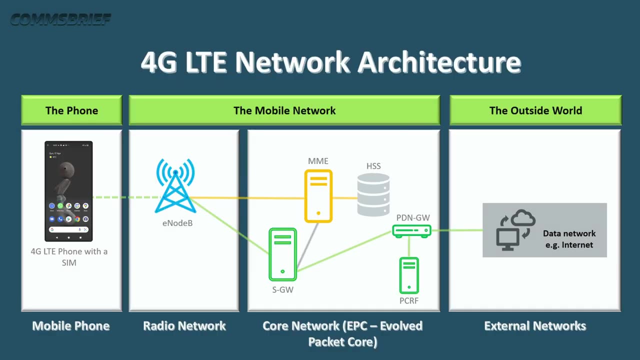 controller. You may recall that in the 2G and 3G networks there is a controller entity in the radio network architecture called Radio Network Controller or RNC, in 3G and Base Station Controller or BSC, in 2G. In LTE we have a base station controller and a BSC. in 2G, We have a base station controller and a BSC in 3G. 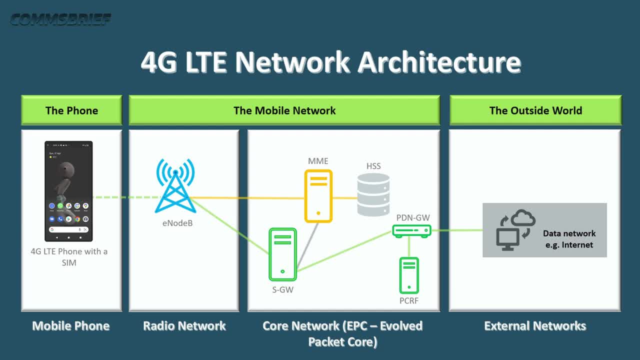 In eNodeB. eNodeB handles both the base station and network controller functions. eNodeB is connected to the Mobility Management Entity, MME, which takes care of all the signaling and exists in the control plane. MME is connected to the home subscriber server, which is the equivalent of HLR. 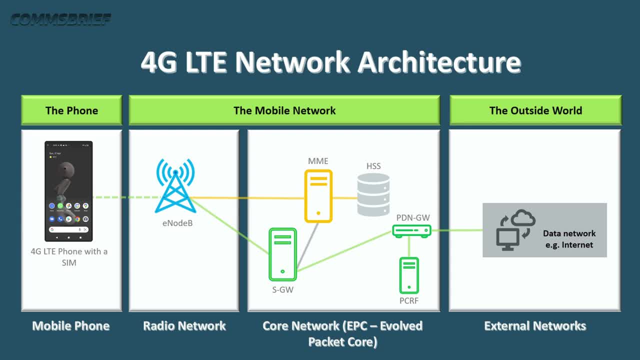 The eNodeB also connects to Serving Gateway or SGW, which is the equivalent of SGSN in 3G. Serving Gateway is in the user plane and is responsible for routing and forwarding data packets. Since 4G LTE is all about data packets, Serving Gateway is the main node that connects the LTE. 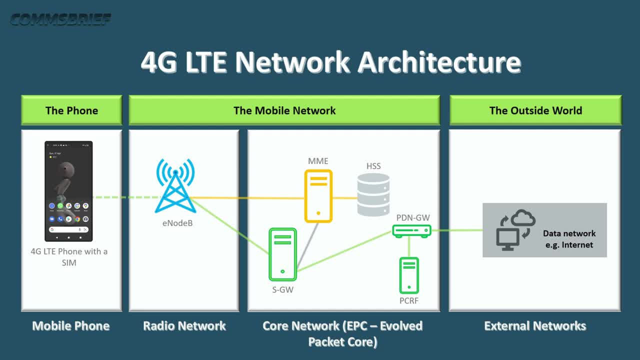 radio network eNodeB to the LTE core network. the Evolved Packet Core or EPC. PDN-GW or Packet Data Network Gateway connects the EPC to outside networks, including the internet. PDN-GW is also connected to the Policy and Charging Rules Function. 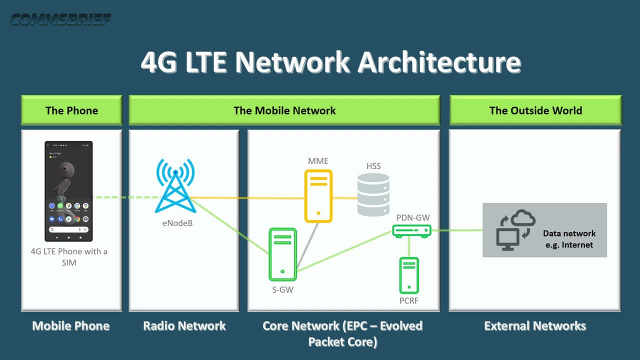 which is a platform where all the business rules reside, So business rules like, for example, how to charge or bill a customer. The EPC works alongside IMS or IP Multimedia Subsystem for Voice over LTE to enable data-based or packet-switched voice calls and text messages. Text messages or SMS, same thing. 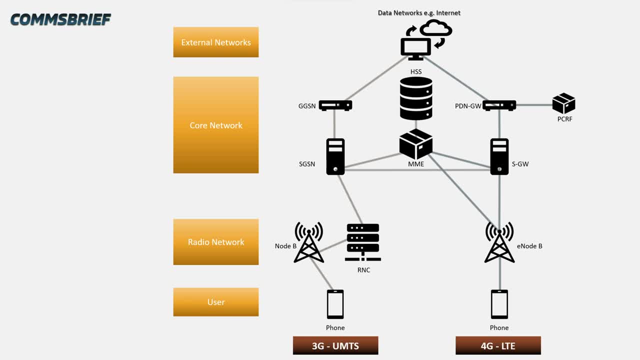 Let's now look at a combined architectural view of 3G UMTS and 4G LTE. As you can see, the eNodeB in 4G is the counterpart of the NodeB and RNC combined in 3G. 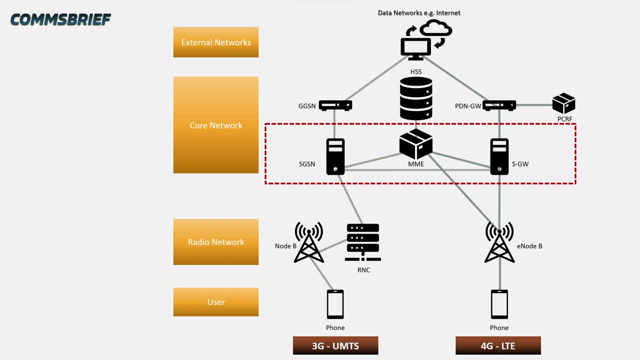 SGW, or Serving Gateway, in 4G is the equivalent of SGSN in 3G. SGSN and Serving Gateway are both connected to MME and are also connected to each other. Finally, PDN-GW in 4G is the equivalent of GGSN in 3G.